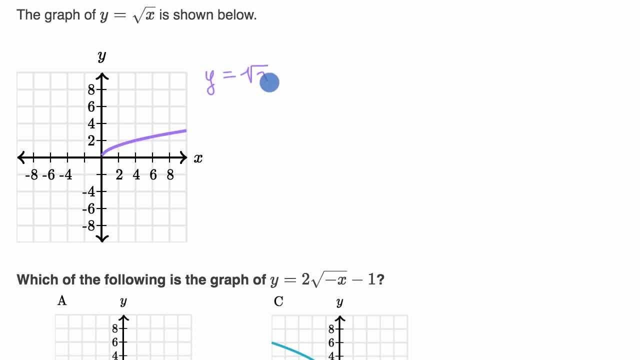 So we already see what y equals. the square root of x looks like. But let's say we just want to build up. So let's say we want to now figure out what is. the graph of y is equal to the square root of, instead of an x under the radical sign. 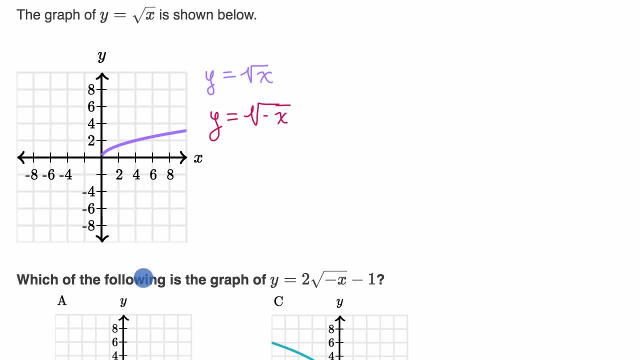 let me put a negative x under the radical sign. What would that do to it? Well, whatever was happening at a certain value of x will now happen at the negative of that value of x. So square root of x is not defined for negative numbers. 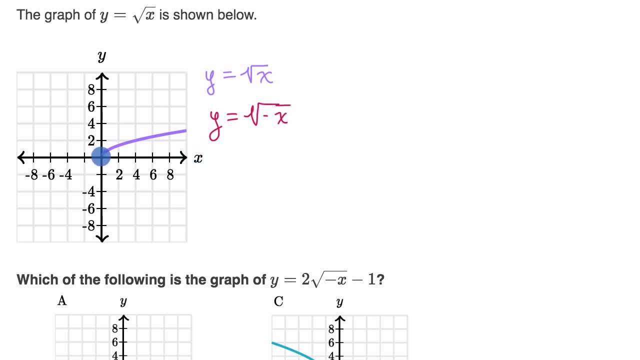 Now, this one won't be defined for positive numbers. And the behavior that you saw at x equals two, you would now see at x equals negative two. The behavior that you saw at x equals four, you will now see at x equals negative four. 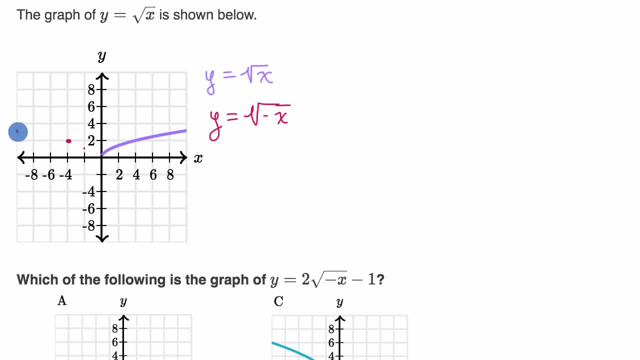 And so on and so forth. So the y equals the square root of negative. x is going to look like this: You've essentially flipped it over the y. we have flipped it over the y-axis, All right, so we've done this part. 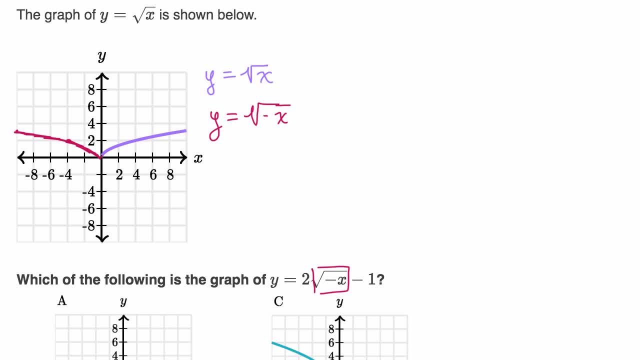 Now let's scale that. Now let's multiply that by two. So what would? y is equal to two times the square root of negative x. look like? Well, it would look like this red curve, but at any given x value, we're gonna get twice as high. 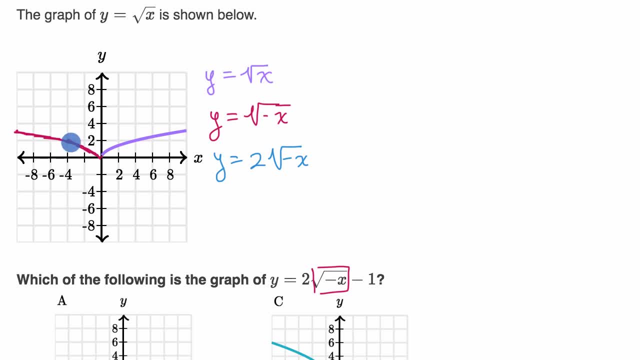 So at x equals negative four instead of getting to two, we're now going to get to four. At x equals negative nine instead of getting to three, we're now going to get to six. Now, at x equals zero. we're still going to be at zero. 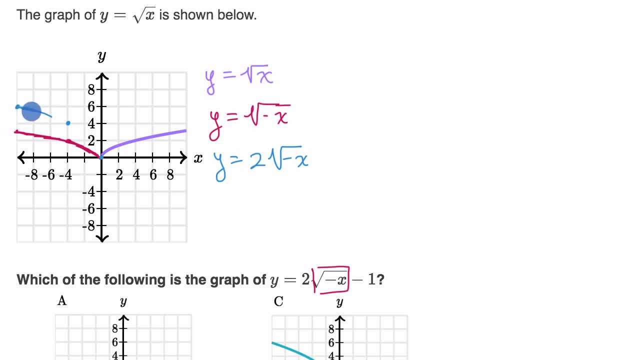 because two times zero is zero. So it's going to look, it's going to look like that, Something like that. So that's, y equals two times the square root of negative x. And then, last but not least, what will y? 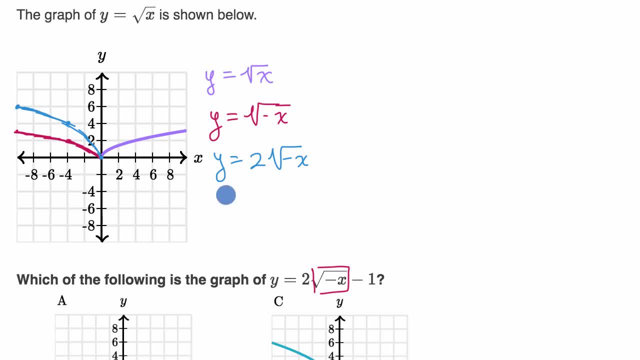 let me do that in a different color. what will? y equals two times the square root of negative x minus one. look like: Well, whatever y value, we're gonna get to same as what we were getting before. we're now just going to shift everything down by one. 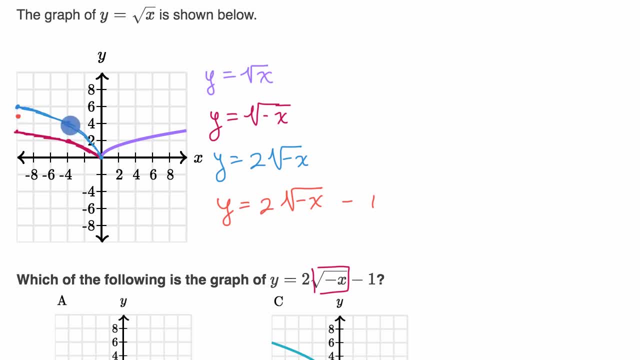 So if we were at six before, we're going to be at five now. If we were at four before, we're now going to be at three. If we were at zero before, we're now going to be at negative one, And so our curve is going to look something like: 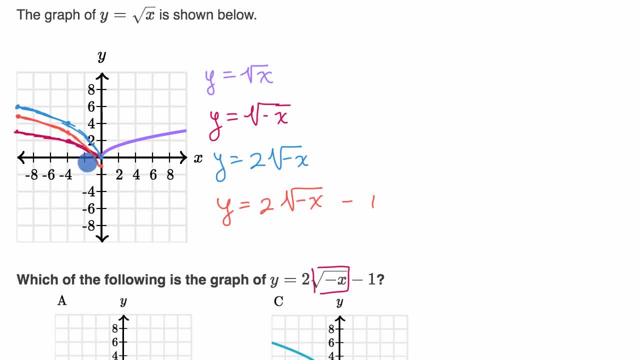 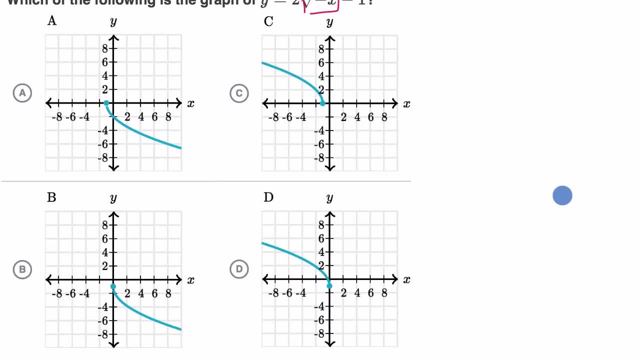 something like that. So let's look for, let's see which choices match that. So let me scroll down here and both c and d kind of look right. but notice, right at zero we wanted to be at negative one. so d is exactly what we had drawn. 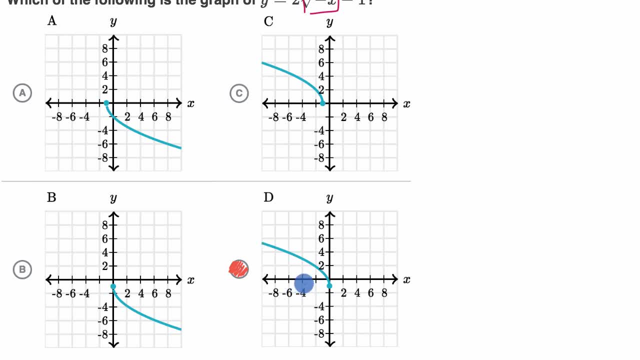 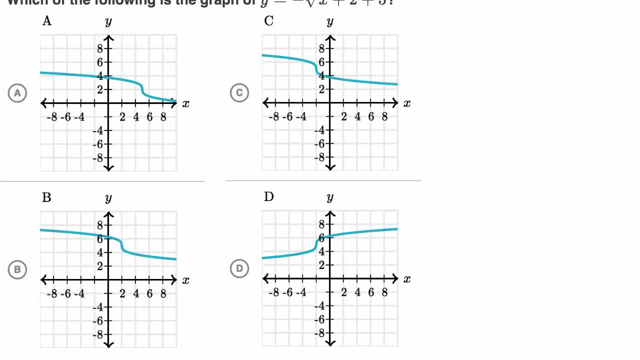 that at nine we're at five, or at negative nine we're at five, at negative four we're at three and at zero we're at negative one- exactly what we had drawn. Let's do another example. So here, this is a similar question. 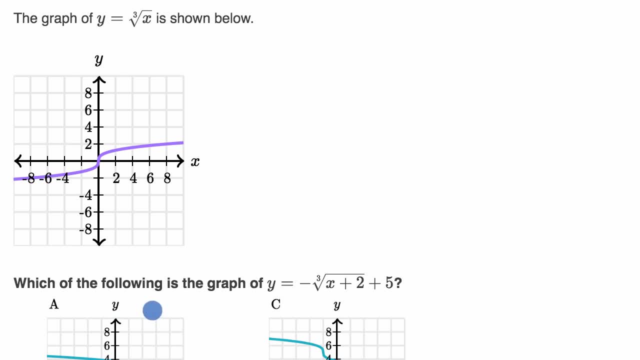 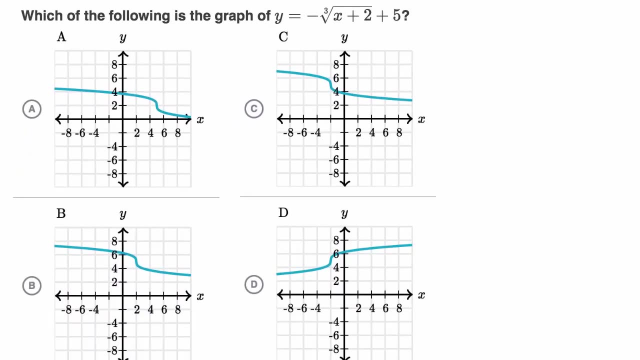 Now they graphed: the cube root of x. Y is equal to the cube root of x. and then they say: which of the following is the graph of this business? And they give us choices again. So, once again, pause this video and try to work it out on your own. 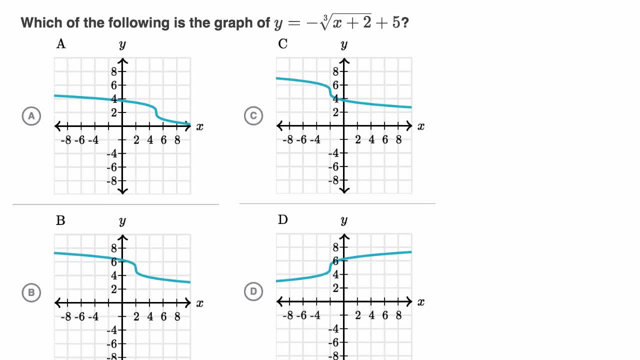 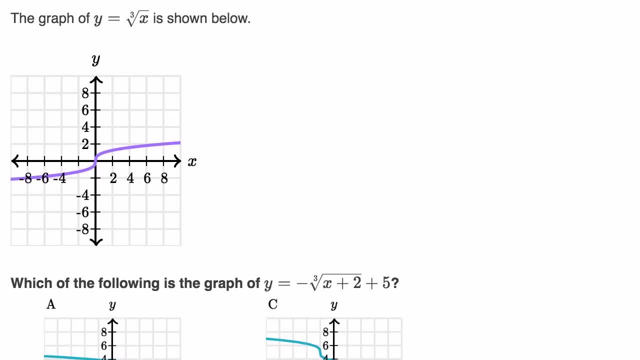 before we do this together. All right, now let's work on this together, and I'm gonna do the same technique. I'm just gonna build it up piece by piece. So this is already. y is equal to the cube root of x. 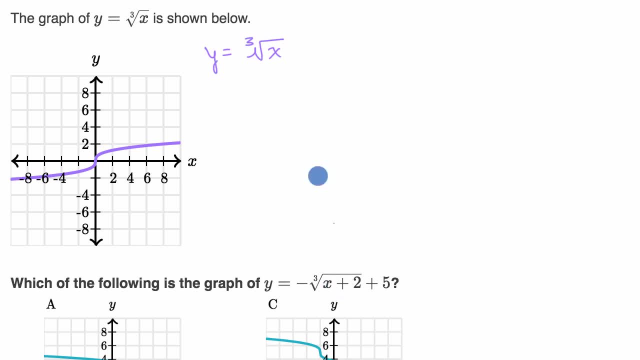 So now let's build up on that. Let's say we wanna now have an x plus one plus two under the radical sign. So let's graph: y is equal to the cube root of x plus two. Well, what this does is it shifts the curve two to the left. 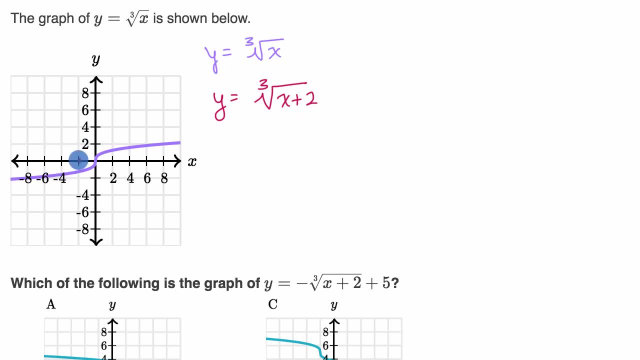 and we've gone over this in multiple videos before. So we are now here and you can even try some values out to verify that At x equals zero. at x equals zero, or actually, let me put it this way- At x equals negative two. 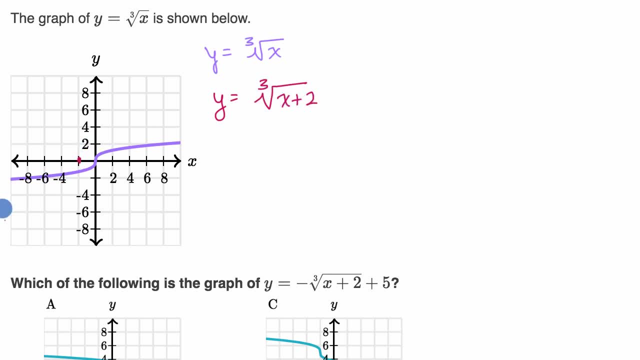 you're gonna take the cube root of zero, which is right over there. So we have now shifted two to the left to look something like this: And now let's build up on that. Let's multiply this times the negative, So y is equal to the negative of the cube root of x plus two. 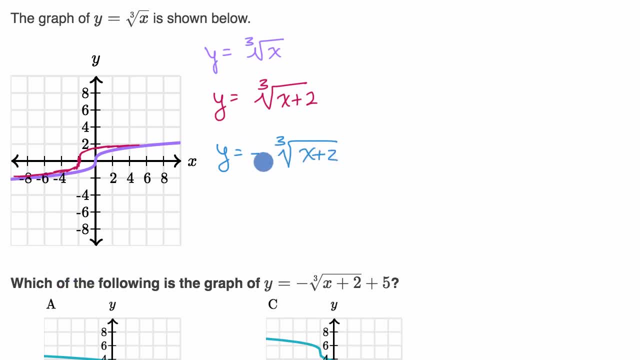 What would that look like? Well, if you multiply your whole expression, or, in this case, the whole graph, or the whole function, by a negative, you're gonna flip it over the horizontal axis, And so it is now going to look like this: